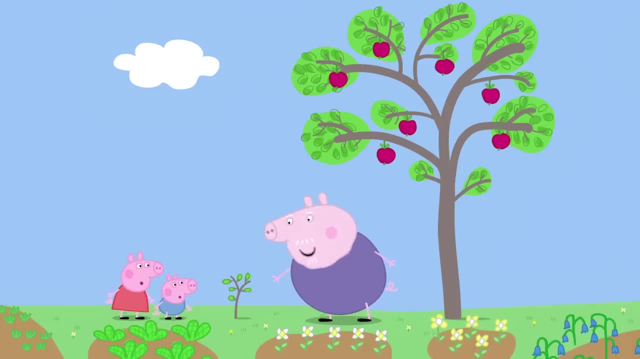 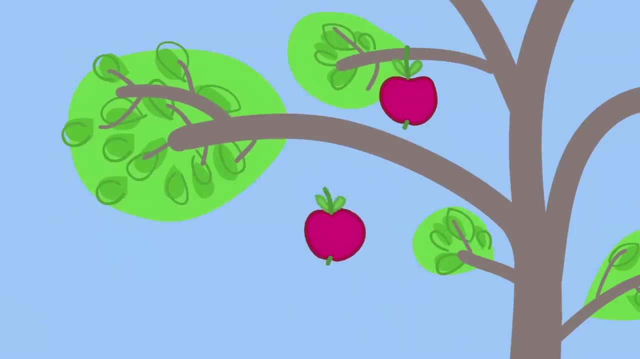 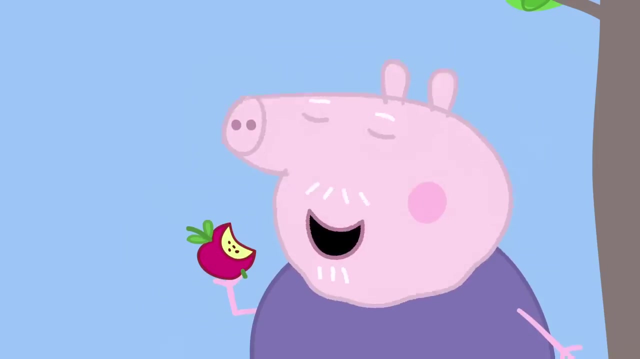 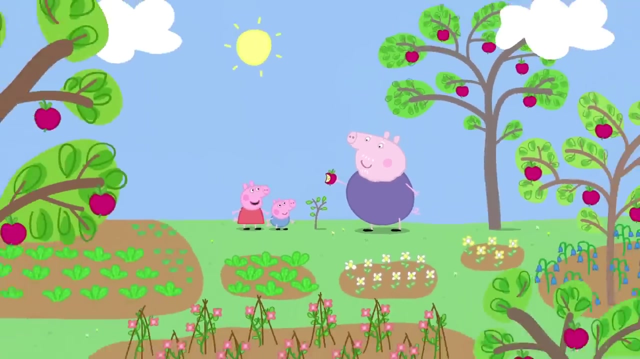 Like this: Ooh, And that little apple tree will grow into a big apple tree. Like this, Like this, Ouch, And inside this apple are more seeds To make more apple trees. Exactly, Grandpa, Grandpa, I want to plant a seed. 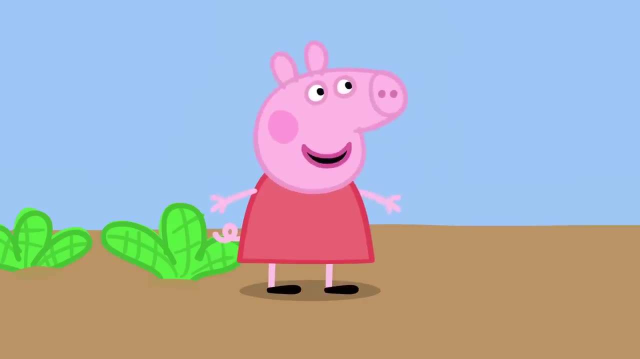 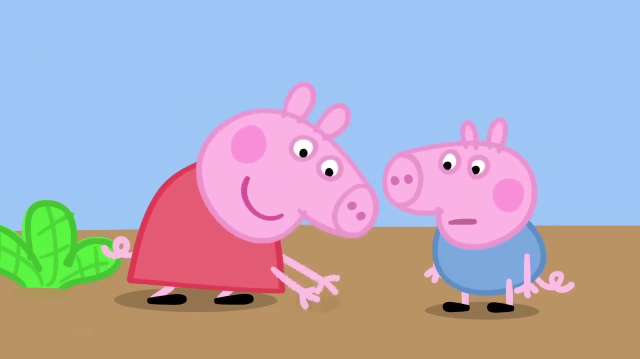 Would you like to plant a strawberry seed? Yes, please. This seed will grow into a- Oh a lovely strawberry plant. First make a little hole, Then I put the seed in And cover it with earth. Shall I water it for you? 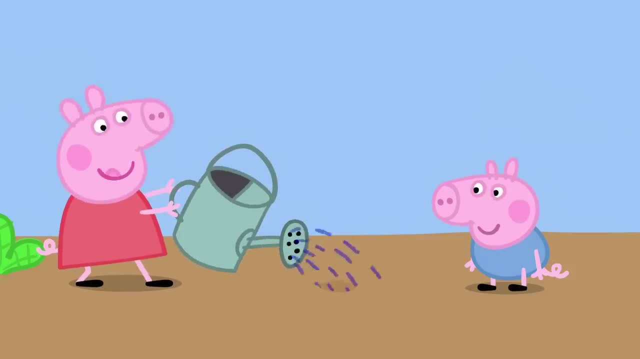 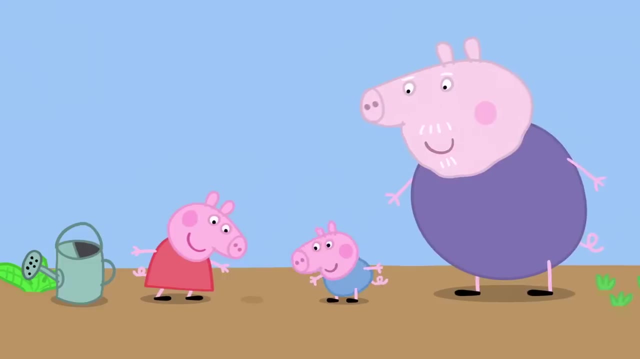 No, no, I want to water it. Good, Now we wait for it to grow. Peppa and George are waiting for the seed to grow. Peppa and George are waiting for the seed to grow. It's not doing anything. 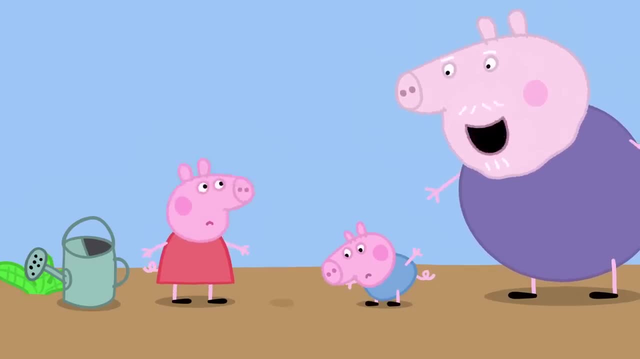 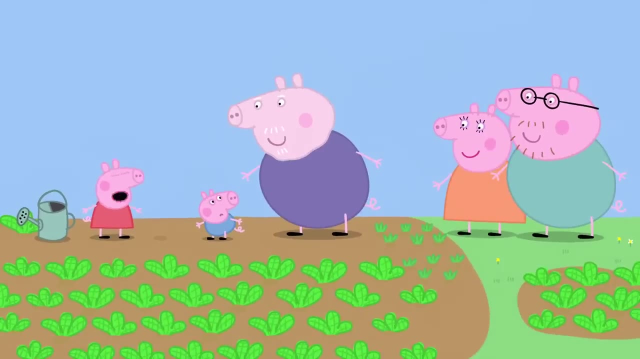 You'll have to be patient, Peppa. It will take a long time to grow. Peppa, George, it's time to go home, But we're waiting for my strawberry plant to grow. I want a strawberry for tea. 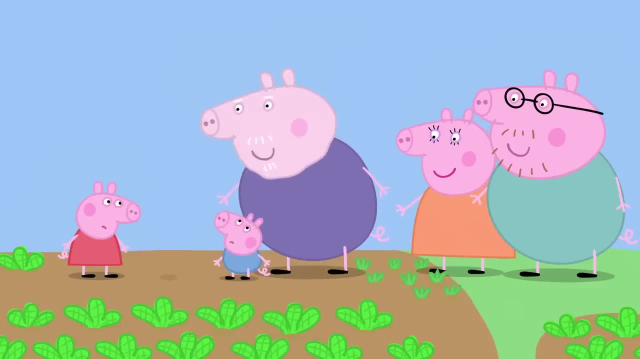 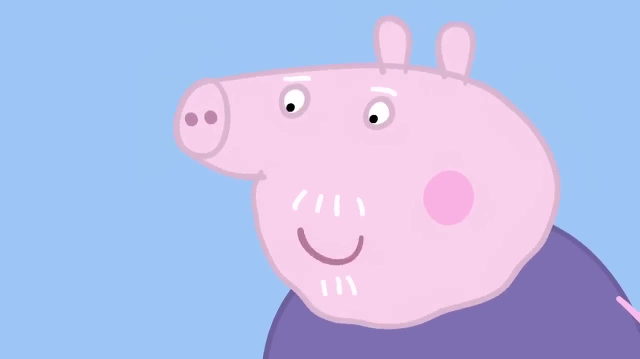 Don't worry, Peppa, Next time you come, the seed will have grown into a plant. I will have strawberries. Yes, Yes, Come on, Peppa. Bye-bye Grandpa, Bye-bye strawberry. 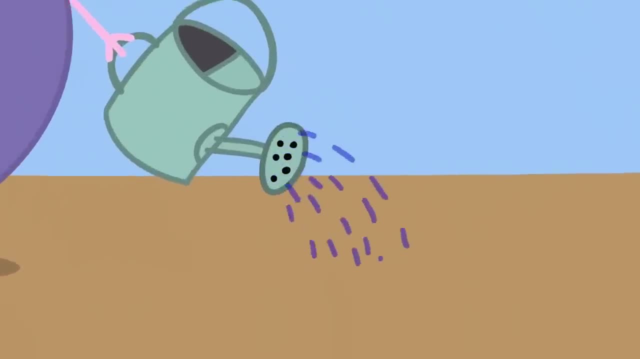 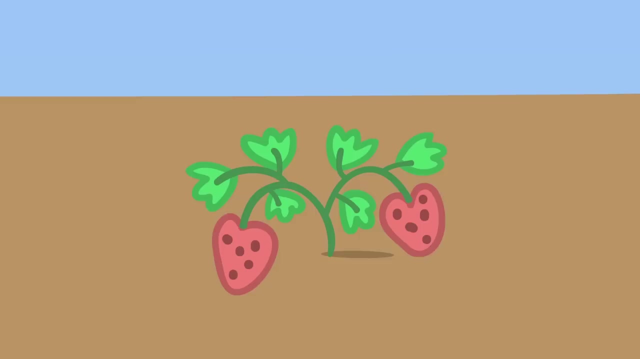 Grandpa Pig looks after Peppa's strawberry plant. After many days, Grandpa Pig finds a tiny plant growing. Day by day, the plant grows bigger and bigger. Then one day Grandpa Pig finds something very special: Strawberries. 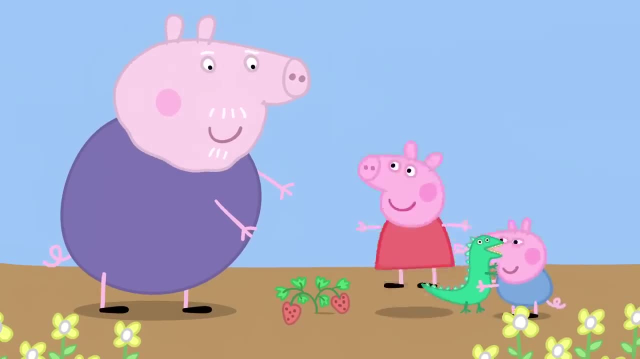 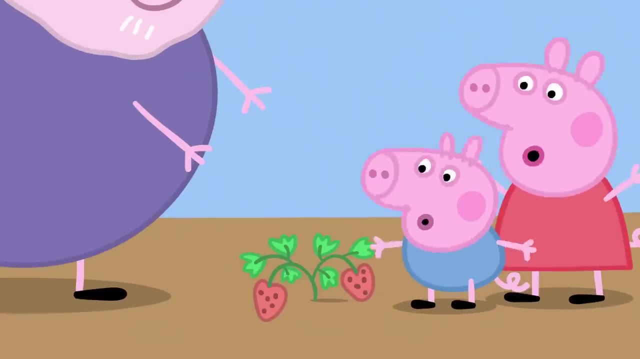 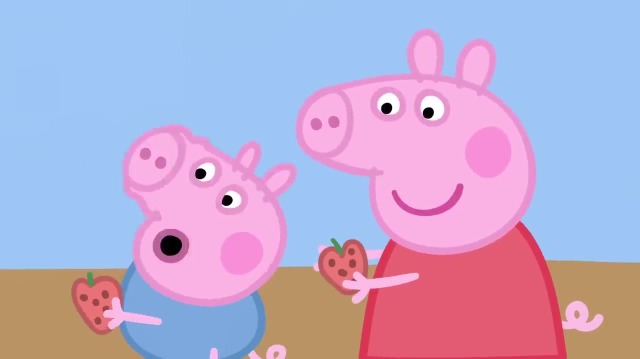 Grandpa, we're back. Peppa and George have come to play again, Grandpa. Grandpa, did my plant grow? Yes, Look Strawberries. Thank you, Grandpa. Thank you Grandpa. Thank you Grandpa.